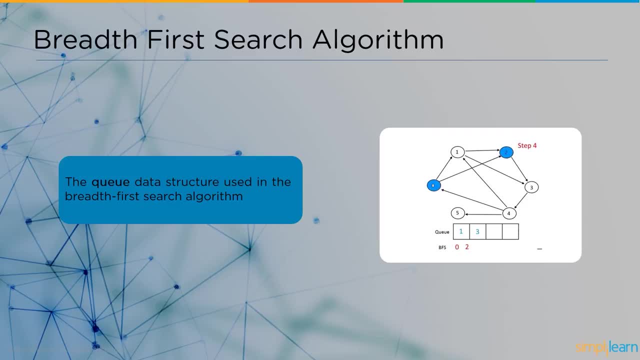 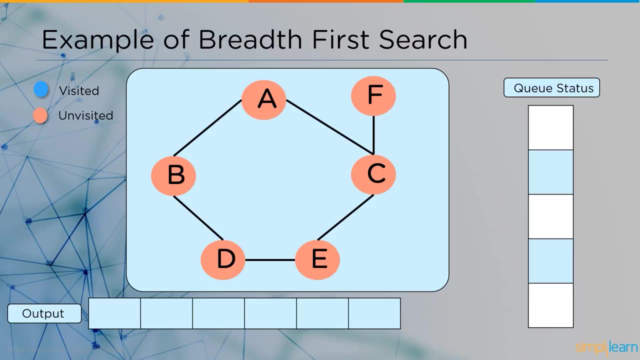 The data structure is used for breadth-first algorithm. For a better understanding, we'll look at an example of breadth-first search algorithm. the blue color indicates that node has been was already explored, while the pink color indicates that the node has not been explored yet. 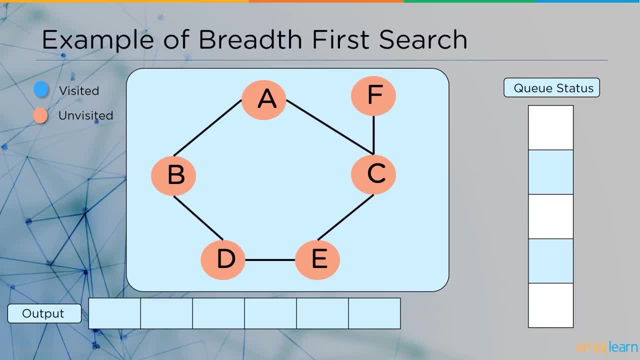 Not visited yet The output. Next we'll have our output. What we'll attach is one thing leading up to this video and the other thing which is nonexistent in. As a result, we'll have node A, which is added to the output and marked as visited. 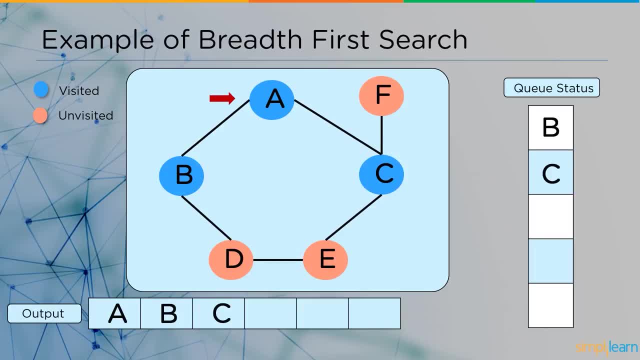 We must verify all the unvisited adjacent nodes of A, that is node B and node C, and add B and C nodes to the output and NQ to the Q according to the breadth first search algorithm. Then we'll look at any node between B and C. We'll start with node B. 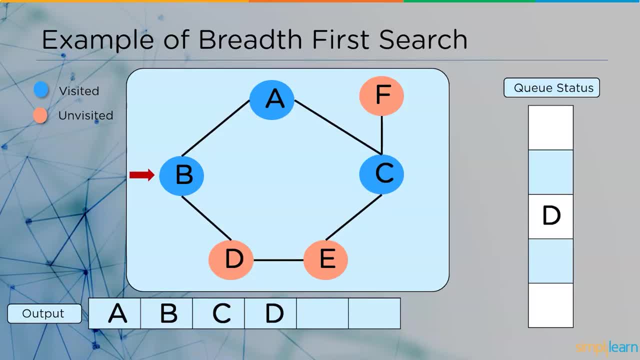 Node D is unvisited, adjacent to node B, so we'll add node D to the output and Q, And since node B is now being visited, we'll dequeue it When it goes to node D. the next unvisited node is node E. 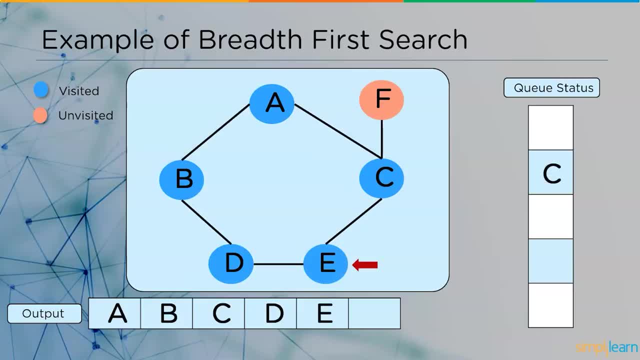 Add node E to the output and NQ to the dequeue Once node D has completed its traversal dequeue from the Q. Now, in the case of node E, the adjacent node is node C, which is already visited. Thus, we will dequeue node C from the Q. 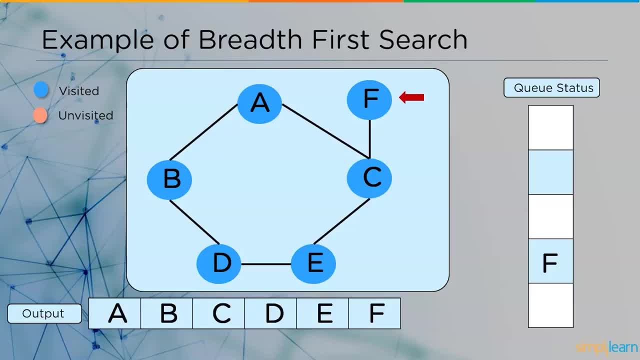 Now that the pointer is pointing to node B and node F is the next unvisited node after the node C, we will set node F to output and Q. Here the pointer leads to node F, which has no unvisited adjacent nodes, So we will dequeue F from the Q and Q is empty. 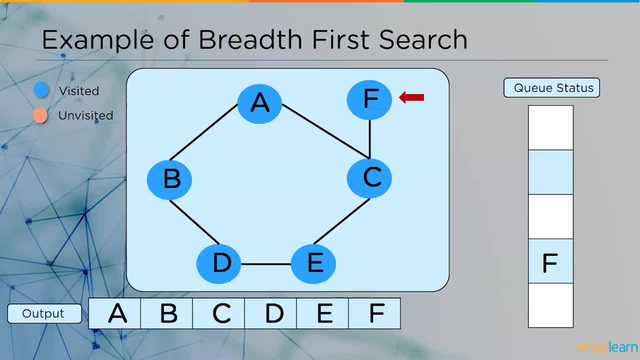 So we'll come to the halt here. Here's what we got, that is, A, B, C, D, E and F. After understanding all the theoretical aspects of BFS algorithm, let's look at the code of BFS algorithm in C programming language. 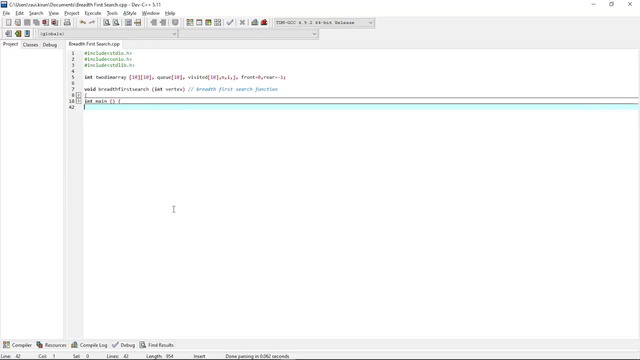 Now we are on the practical mode. On my screen you can see an example for BFS algorithm. We have declared a two-dimensional array with maximum row and column size of 10 and two arrays. The first one is a square of a maximum size of 10 and the second one which is a visited. 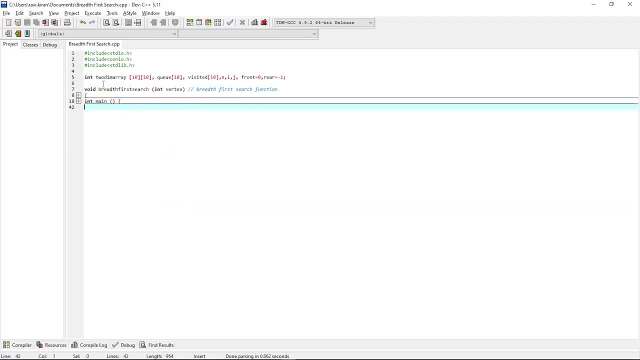 that stores the maximum size of 10, as well Some variables, NIJ and finally, we declared front, which is initialized with 0, and rare variables, which is initialized with minus 1.. We perform a loop from index 1 to the size of an array visited in this function, with the condition: 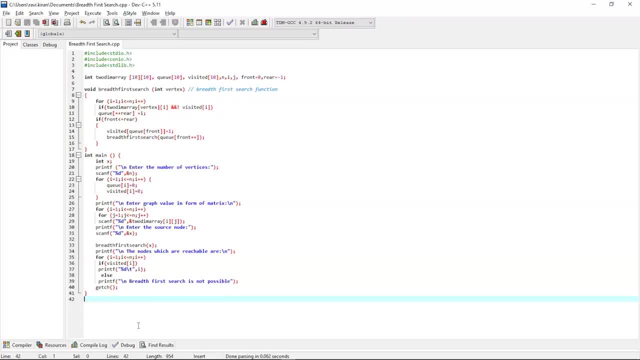 that if two-dimensional array of column 1 and visited array of index is not 1. We initialize variable i to the front of the queue. Then 1 is set as the front of the queue index of the visited array and we use the breadth first. 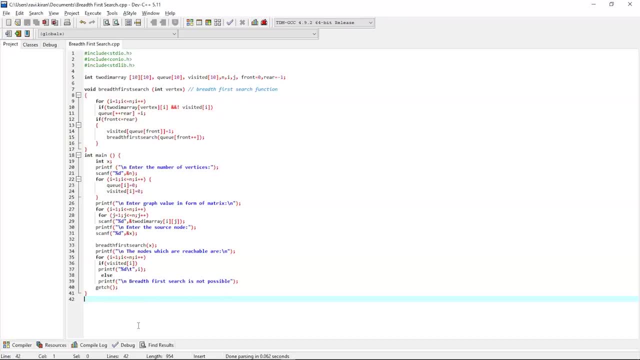 search function with the vertex as the front of the queue, until front is less than or equal to rare. Then we enter the main function Where we define the variable x that stores the graph's vertex, and then we use the printf function to enter the number of vertex that will be stored in variable n. 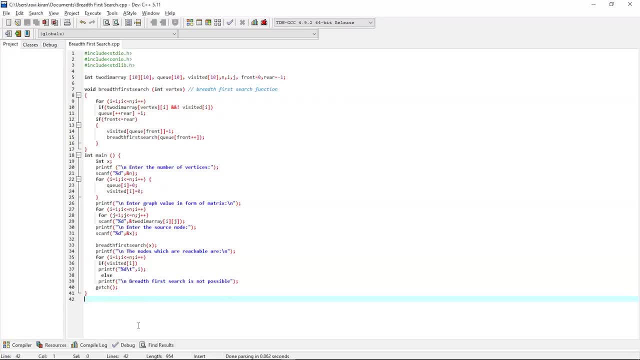 Then we perform a loop from index 1 to queue size and visited array, In which we initialize 0 to the queue and index 1 to the visited array. Then after that, we'll enter the graph value in the form of matrix of two-dimensional. 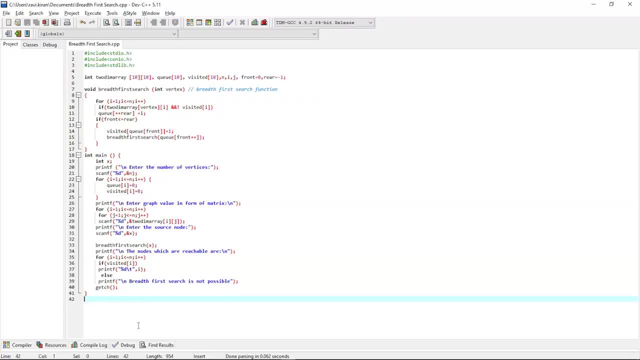 array by performing the loop with two variables: i for the graph row and j for the graph column. Then we print the source node which is saved in the variable x. Then we print the source node which is saved in the variable x and we call the breadth first. 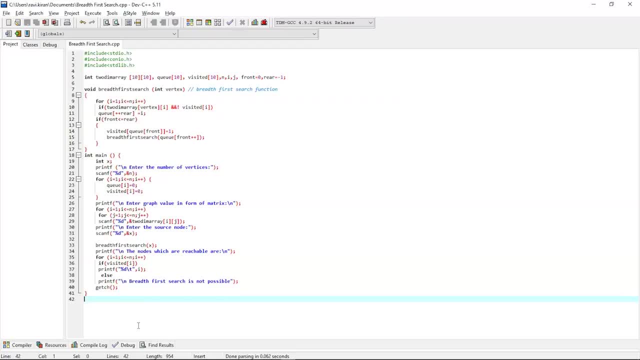 search function or method which takes a vertex x as parameter and we print which nodes are reachable by looping from index 1 to the size of the visited array If index 1 of the array is visited. otherwise, breadth first search is not possible. So this was the explanation of the program. 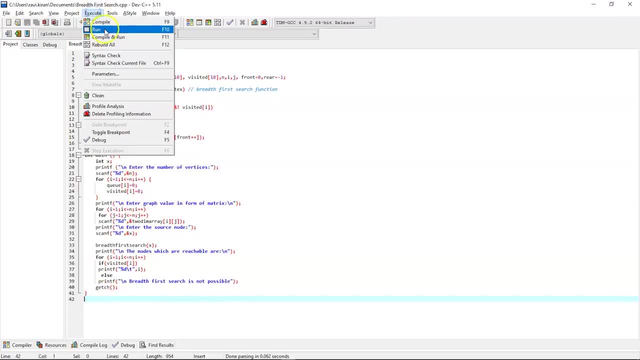 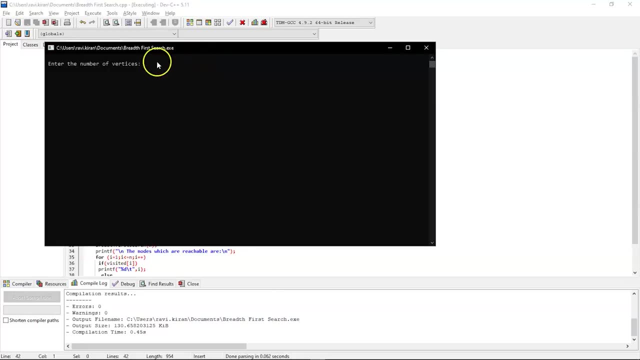 Now let's try to solve the problem. Let's try to execute and see the output. There you go. The program got successfully compiled and now it's asking for the input. Now it is asking for the number of vertices. Let's enter the number of vertices as 3.. 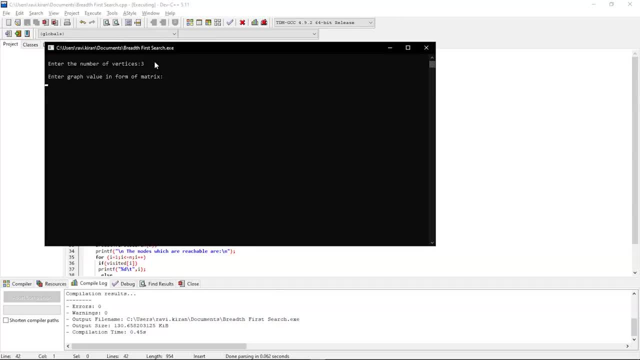 Now it is asking for us to enter the input in the form of matrix. So the first row will be 1, 2 and 3.. So these are the first rows. The next rows will be 2, 3. And 4..